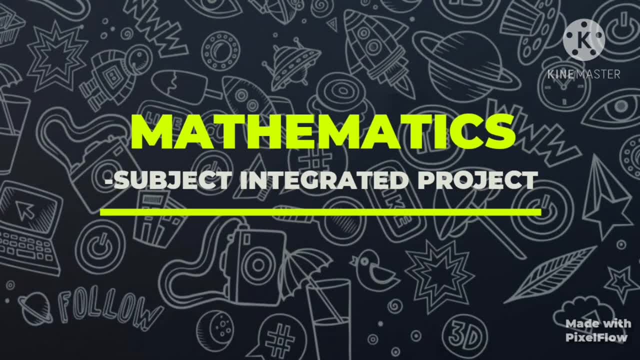 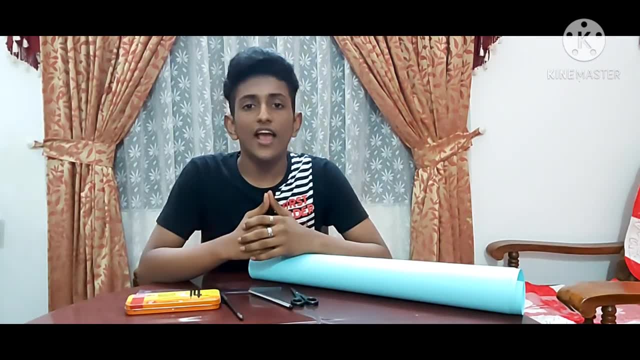 Hi guys, welcome back Myself, Ashish Sundar, student of class 10 of Maharashtra Seed and Seed Industry School. Today I am going to demonstrate a video on the relationship between volume of cylinder and volume of foam. Friends, you all must be familiar with the formula for finding volume of cylinder. 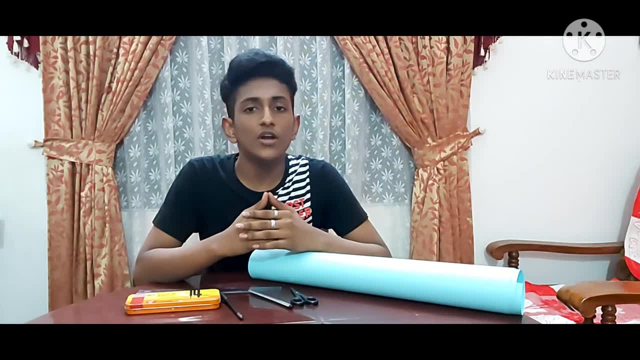 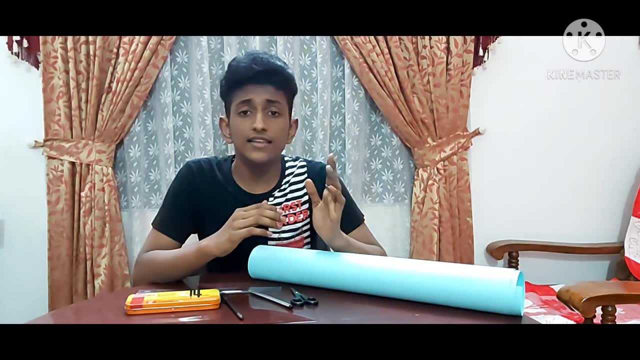 It is pi r squared, while the formula for finding volume of foam is 1 by 3 pi r squared. From these two formulas we can understand that volume of cylinder is 3 times the volume of foam. has the same radius and height. 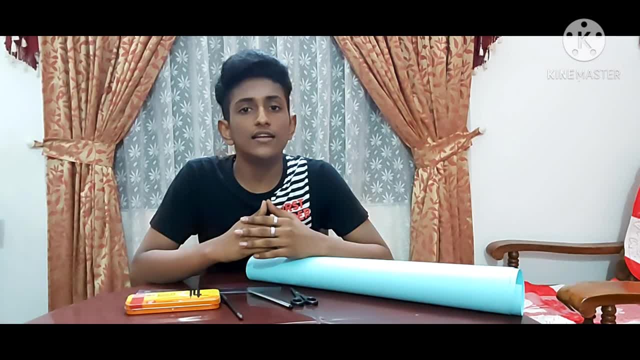 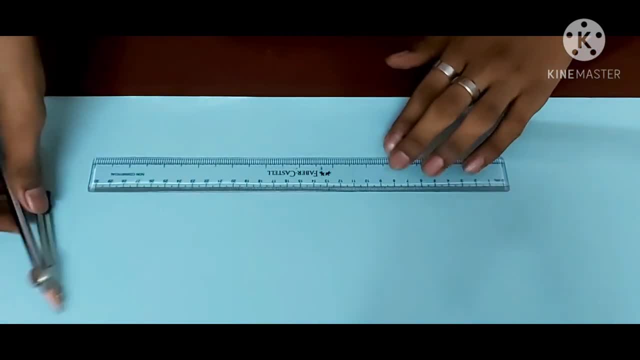 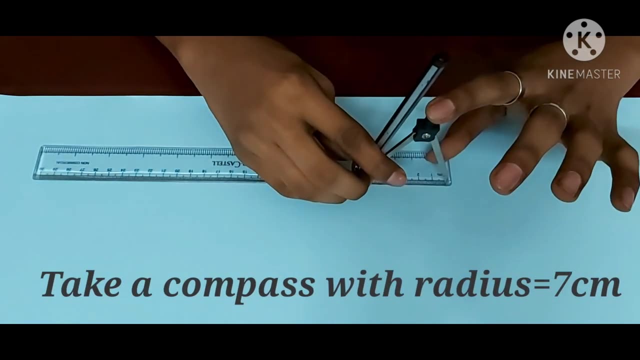 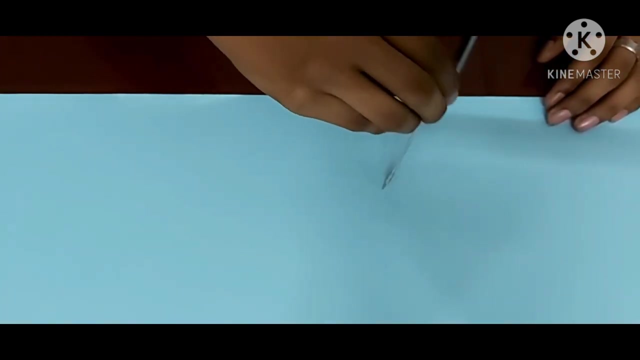 In this video I am going to demonstrate how to make cylinder and cone of same height and radius and how it satisfies the purpose. It is 2 pi r squared and 2 pi r squared of the function of volume, inspired in the previous video. 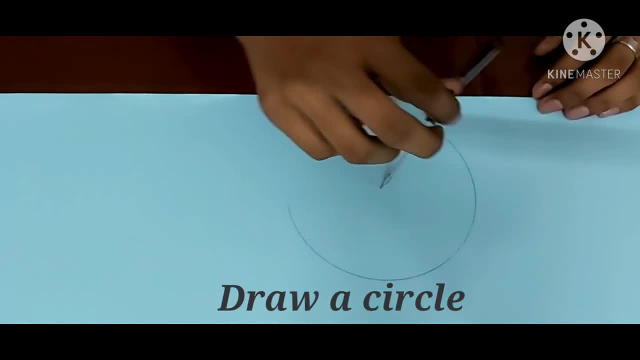 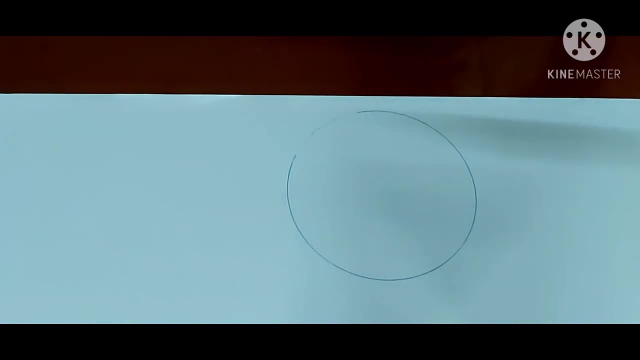 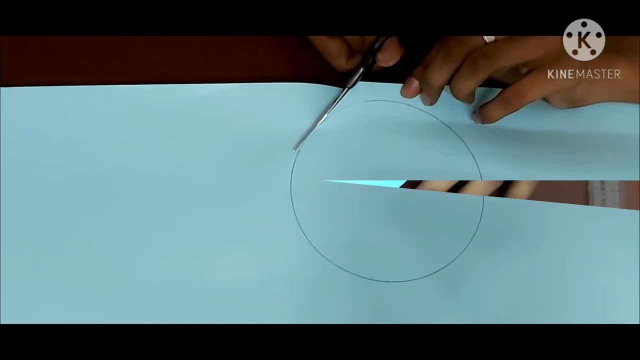 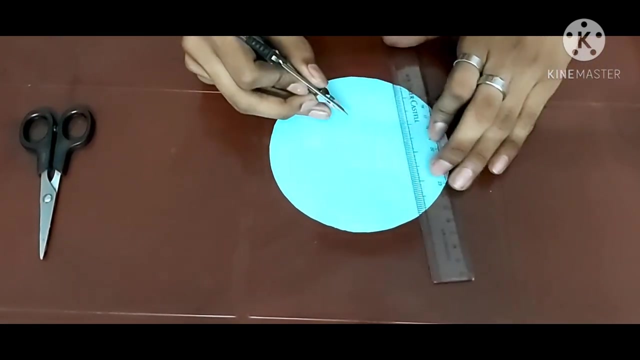 Here we have 2 pi r squared and 2 pi r squared of an. There is a triangle shape on the image. Theorrow we have lower should be the doubling over which we gonna be adding voice input From here. it isumbt until one by two pieces of the same volume. 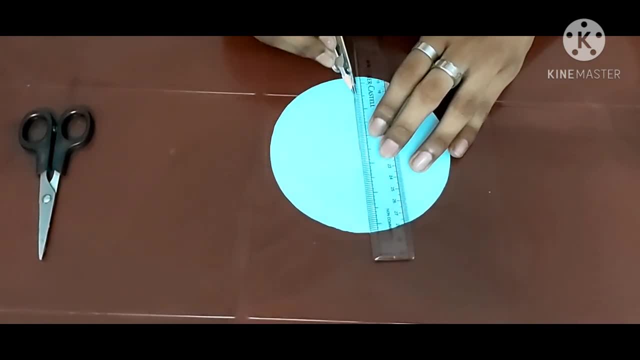 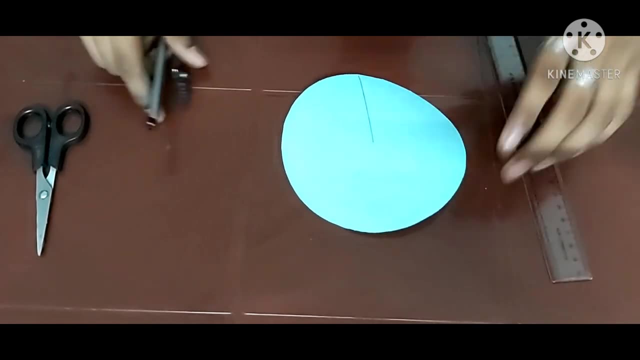 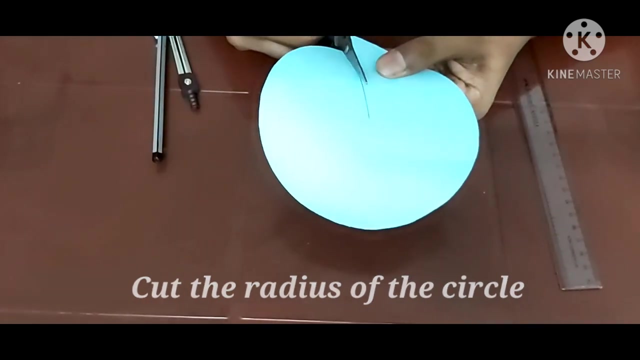 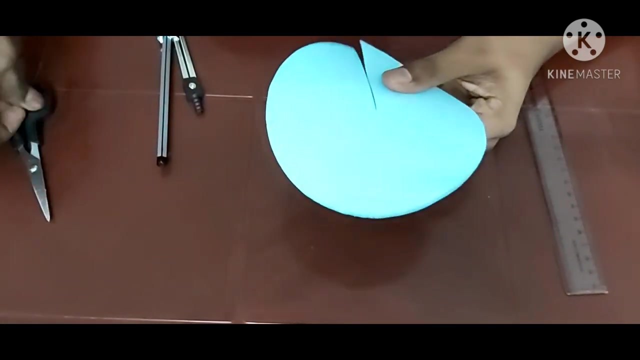 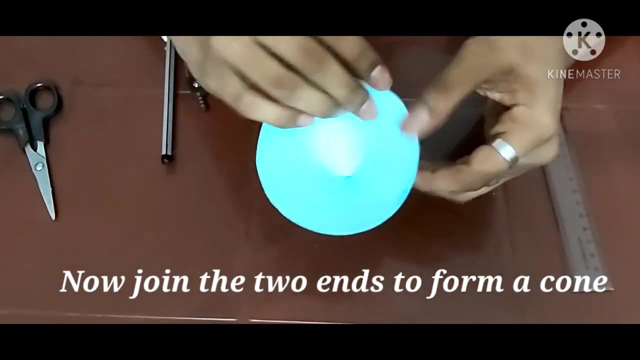 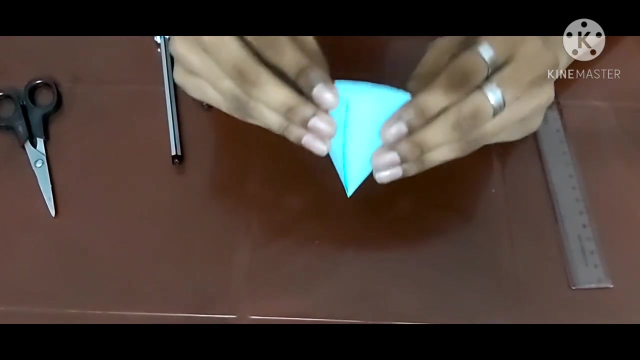 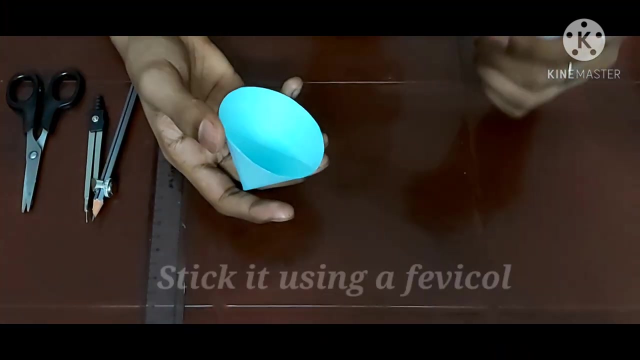 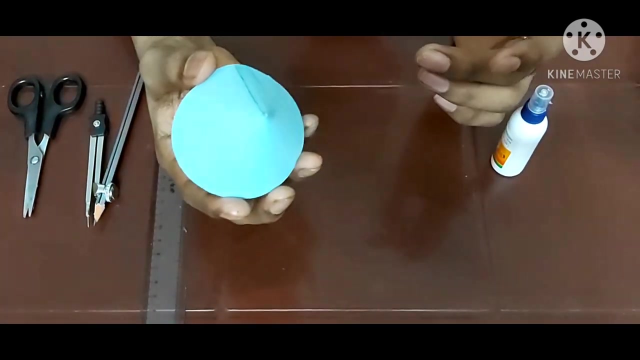 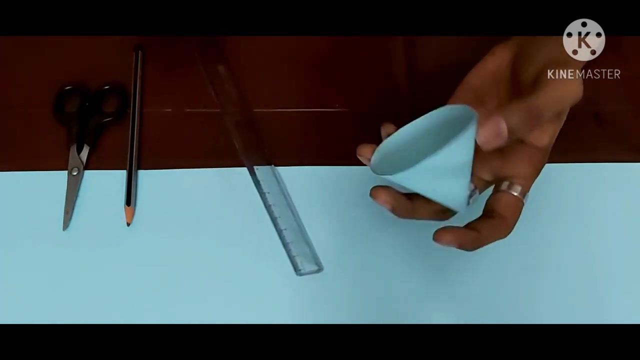 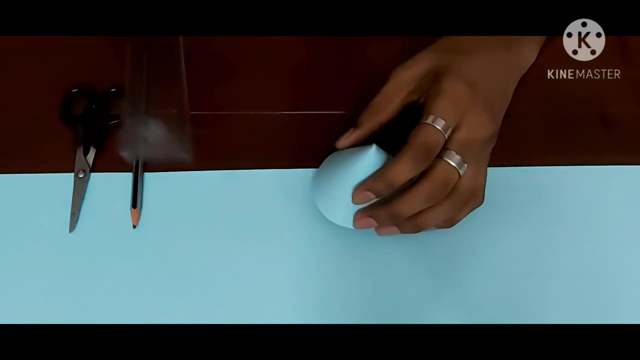 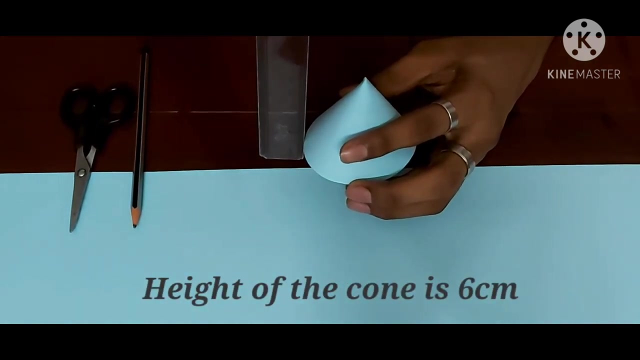 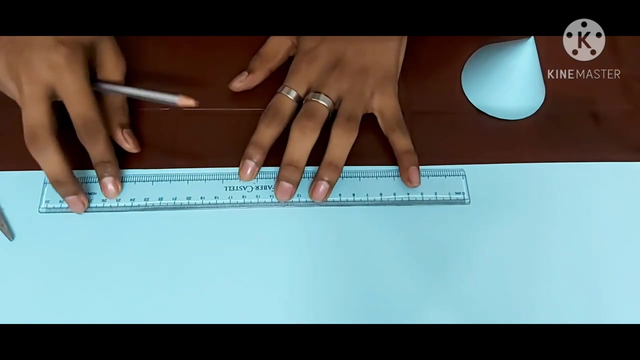 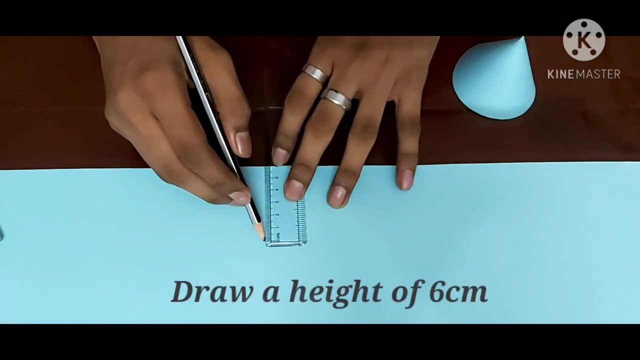 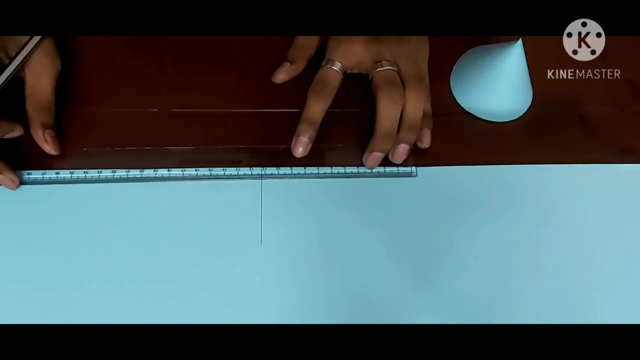 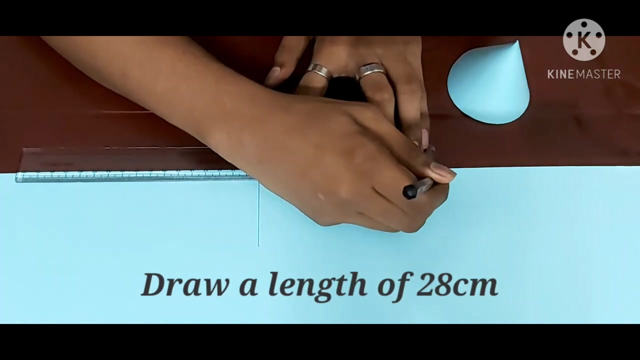 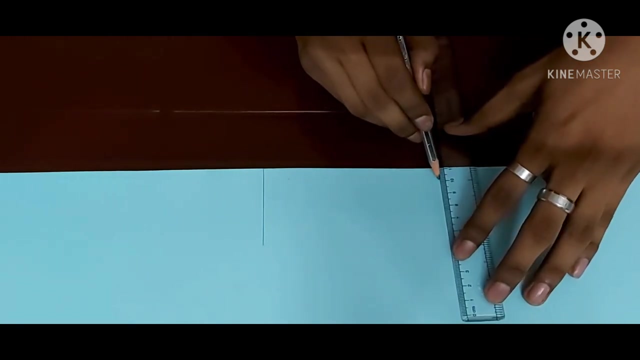 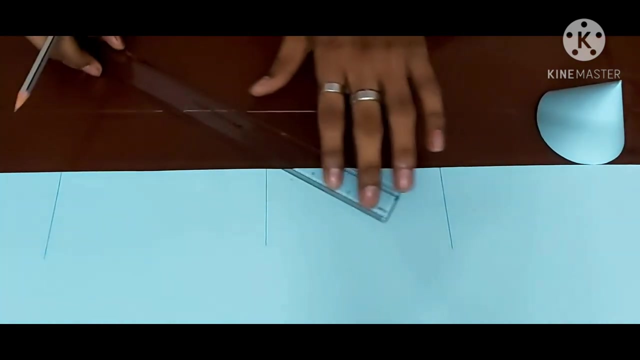 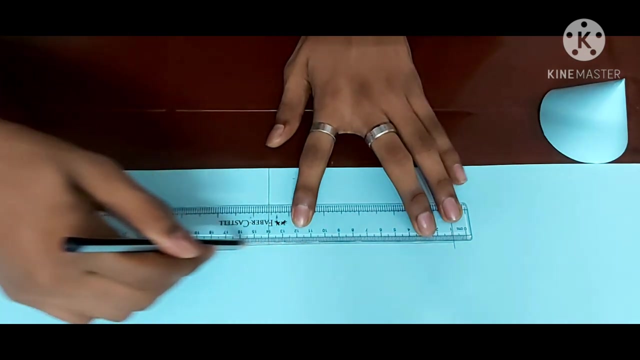 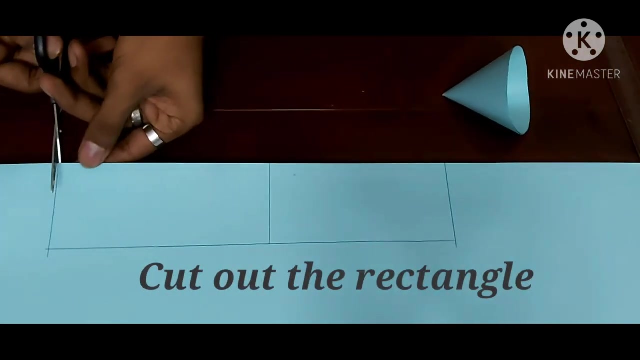 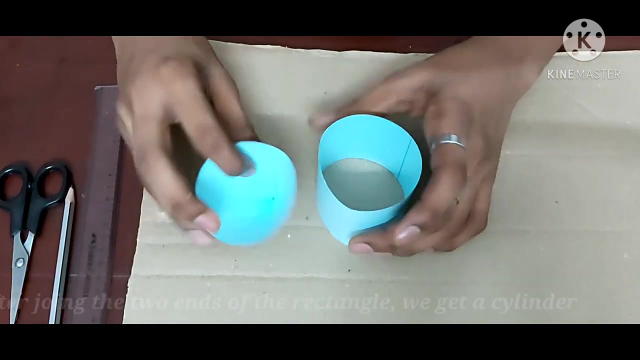 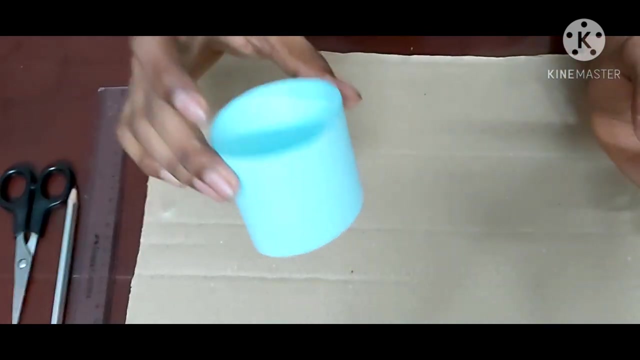 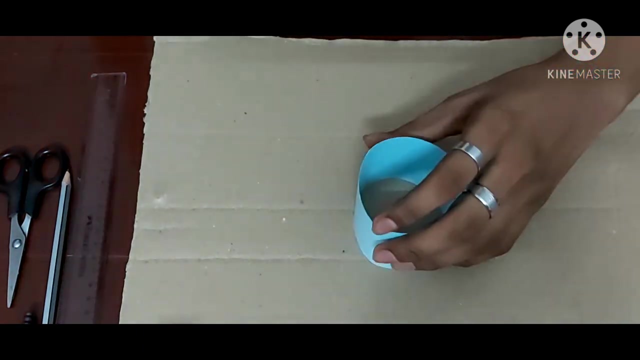 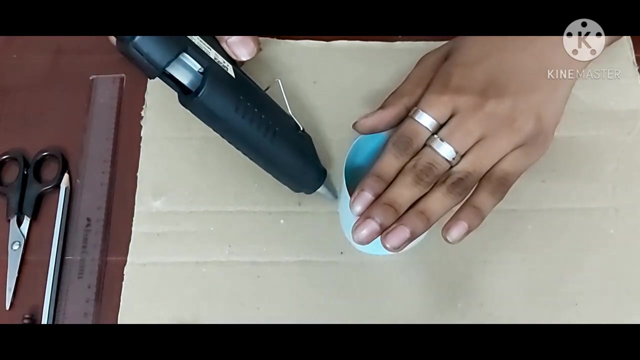 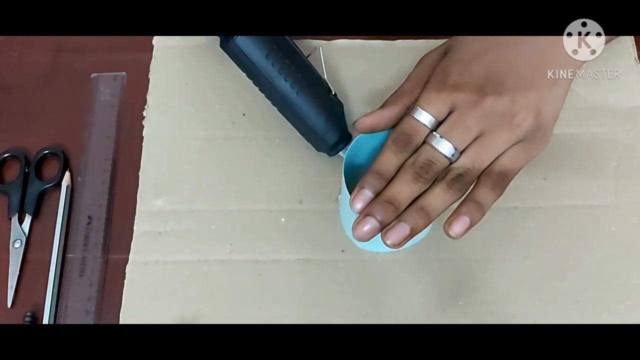 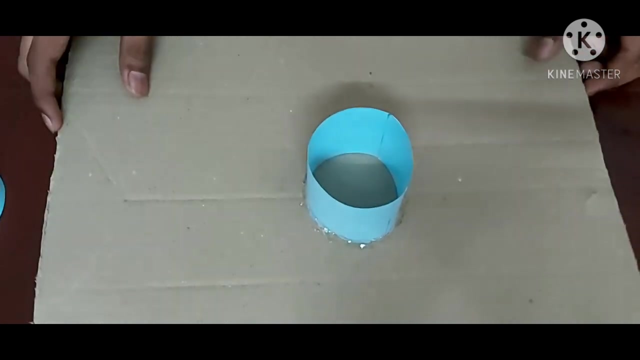 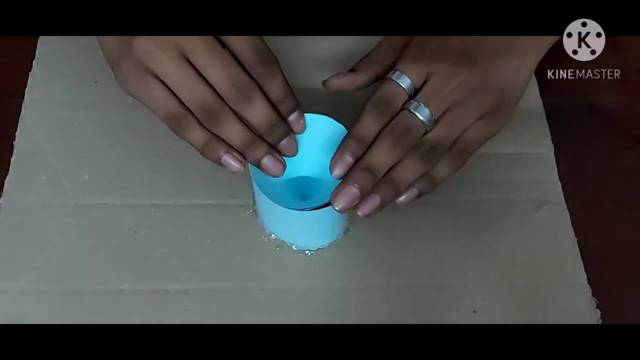 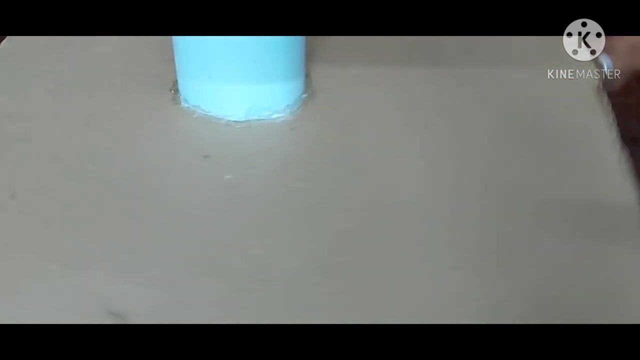 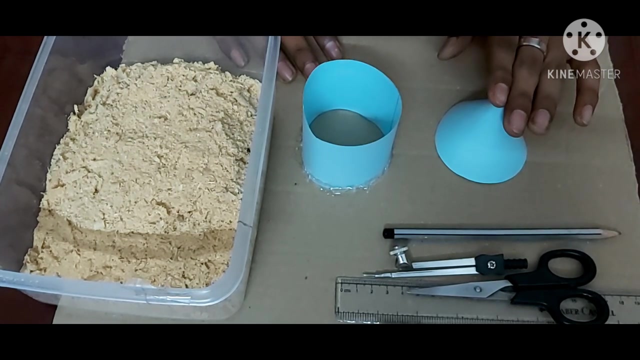 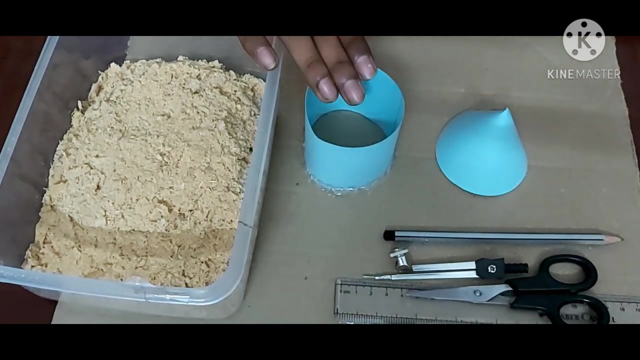 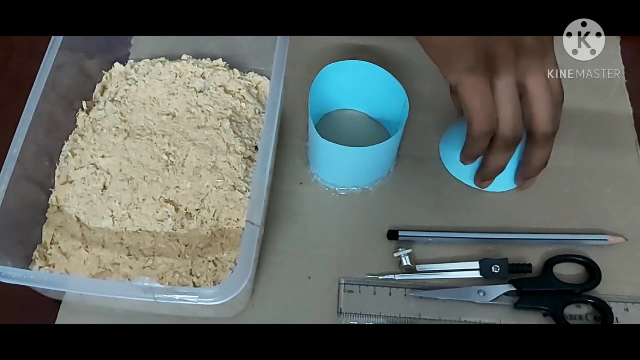 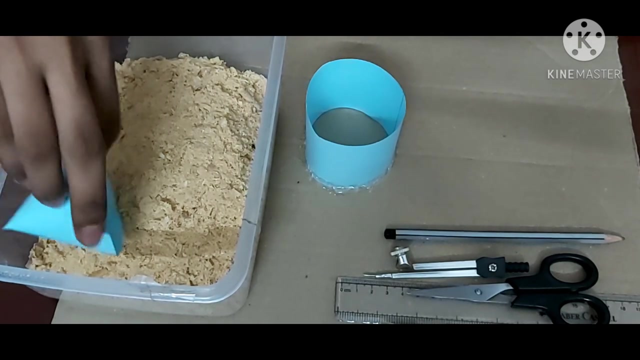 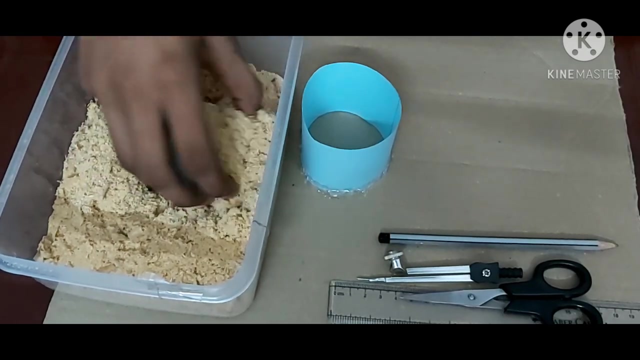 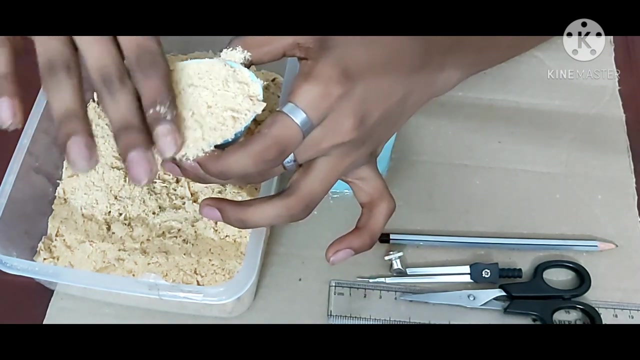 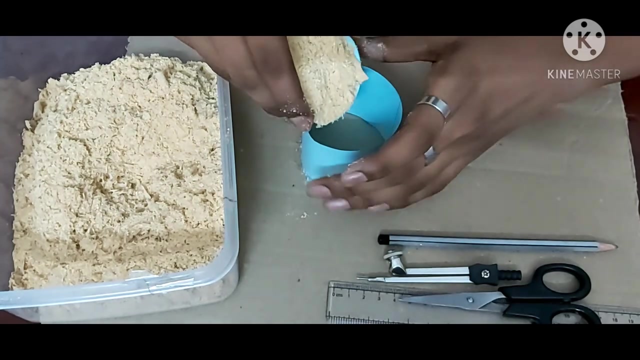 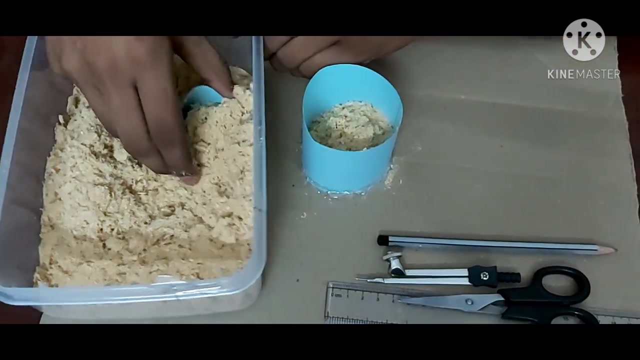 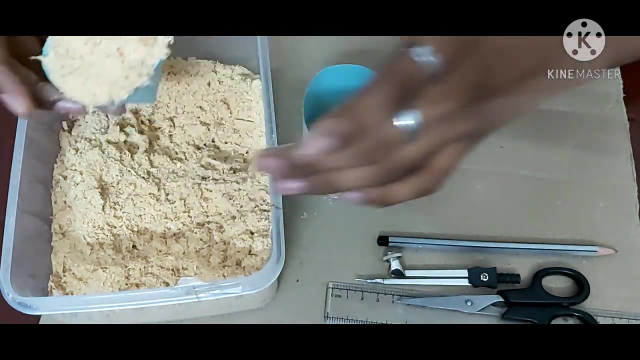 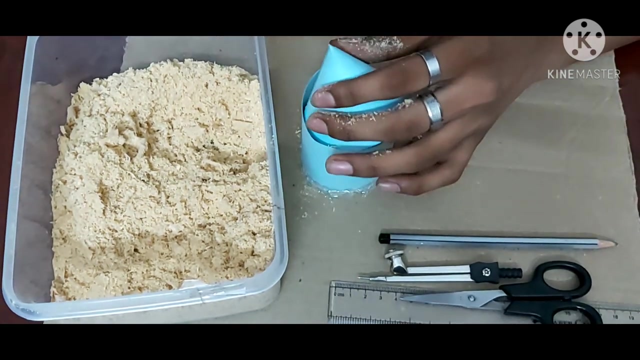 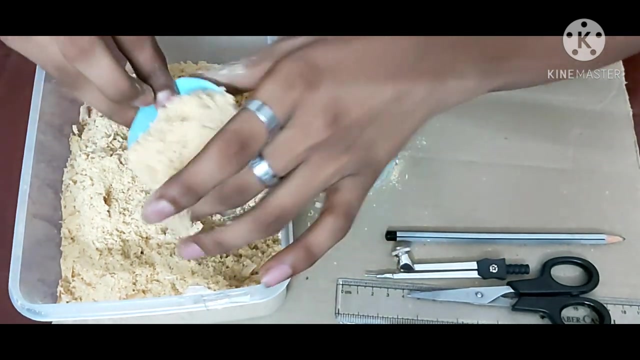 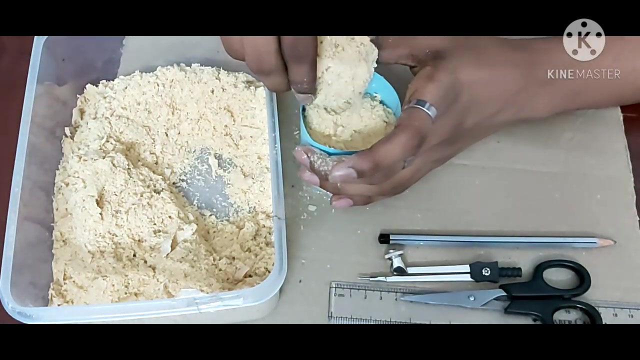 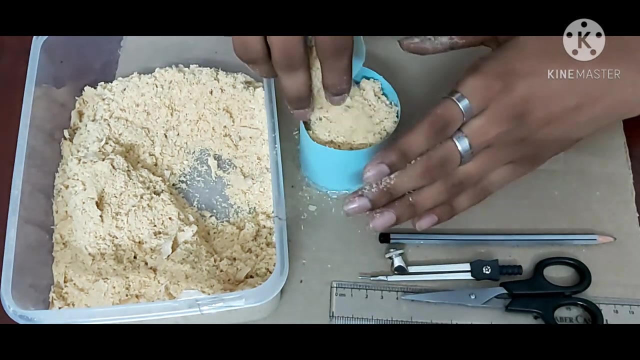 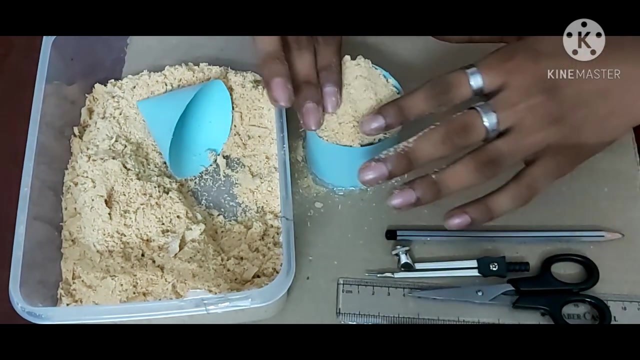 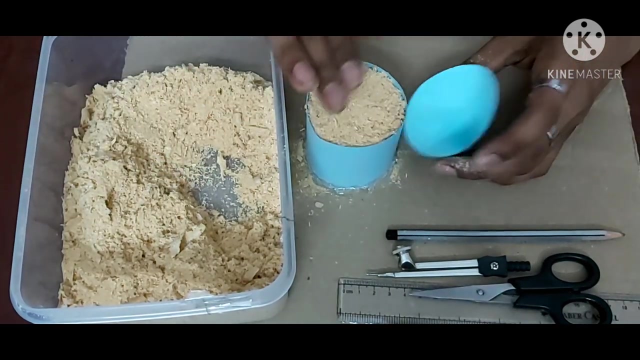